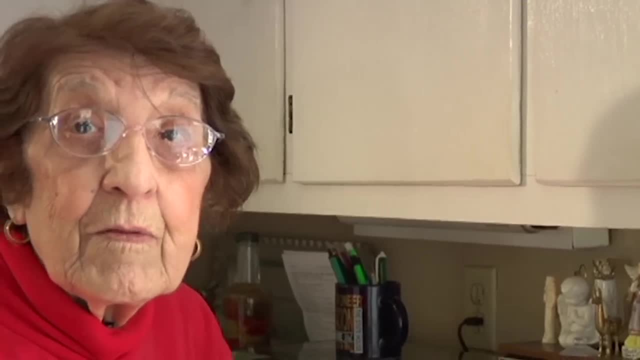 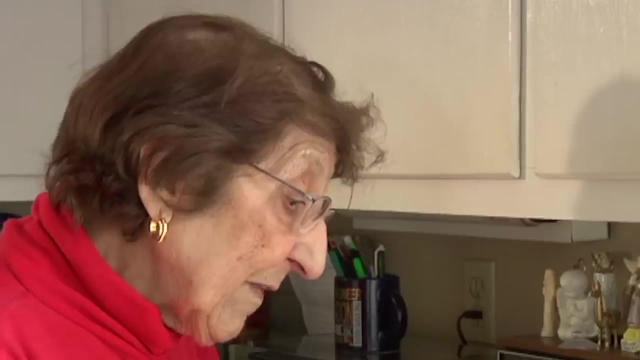 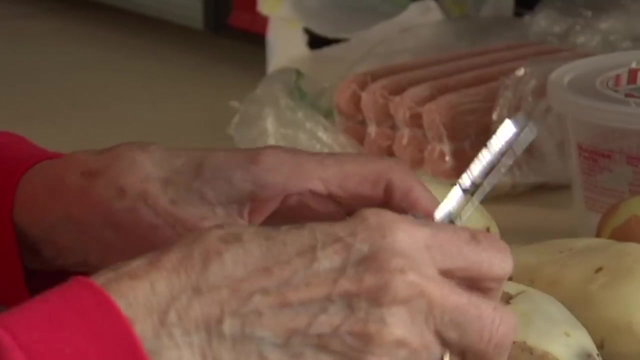 My father would buy a sack of potatoes, a sack of everything flour Potatoes were a dollar a sack. That was a lot of money- a dollar. This is the last one I think I'm going to peel. I think today the kids like this meal. My grandson's like it. 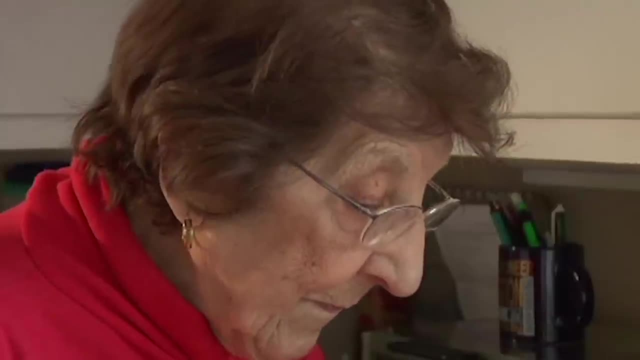 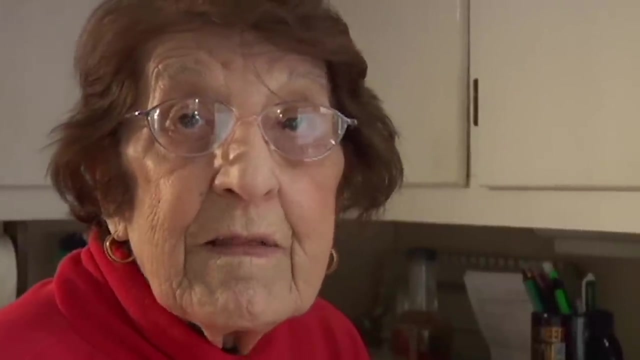 His friends like it. They come here for a poor man's meal. If we had a bad potato, we'd take the best part out and still eat it. If we had a bad potato, we'd take the best part out and still eat it. 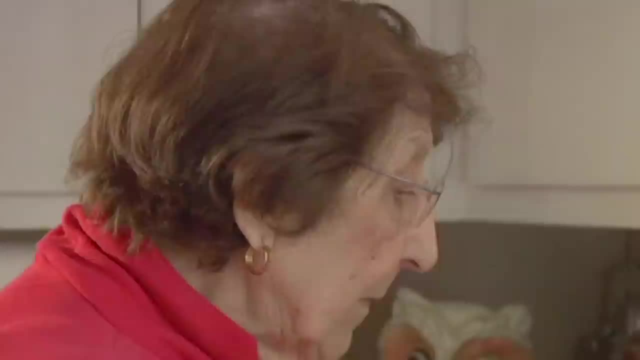 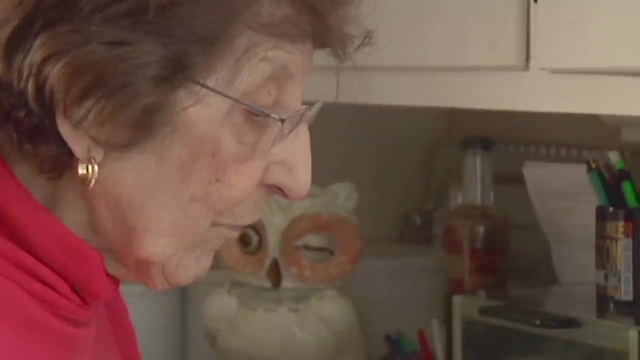 The next step is to cube the potatoes. After you peel them, you cube them, Take out all the bad parts. You know I had to quit high school because I didn't have socks to wear. You know I had to quit high school because I didn't have socks to wear. 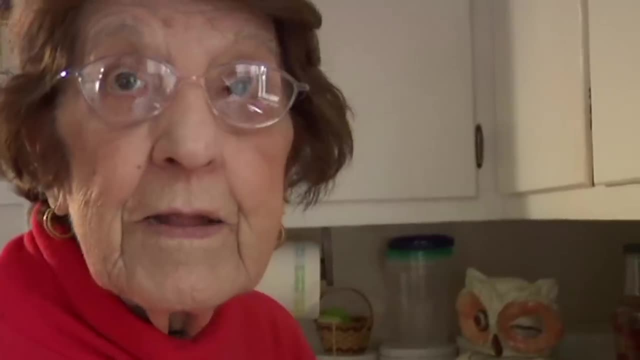 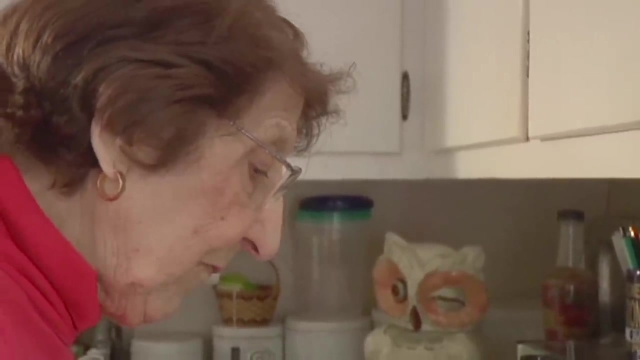 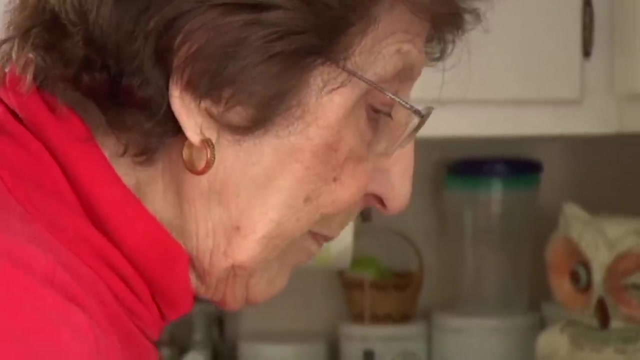 That's a fact. Now I'm putting the onion in the potatoes. Well, it all depends on how many potatoes you have, And I think this, in this case, one onion- is enough. Now I'll put a little oil in the pan. 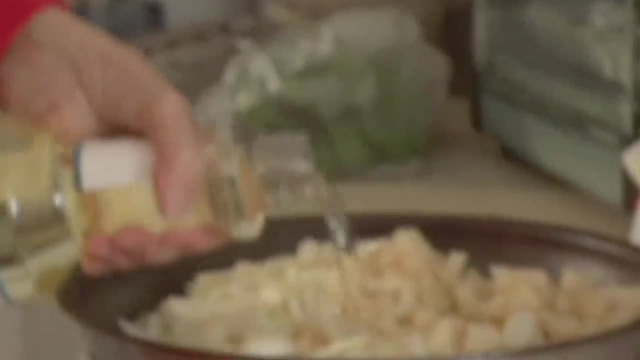 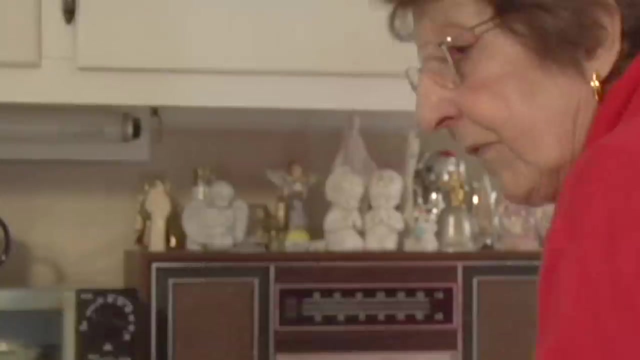 Just judge by yourself how much oil you need. If it runs out of oil, you put a little more, But in this case we don't know yet. So I'm going to put this on the stove now and fry them. So turn on the gas. 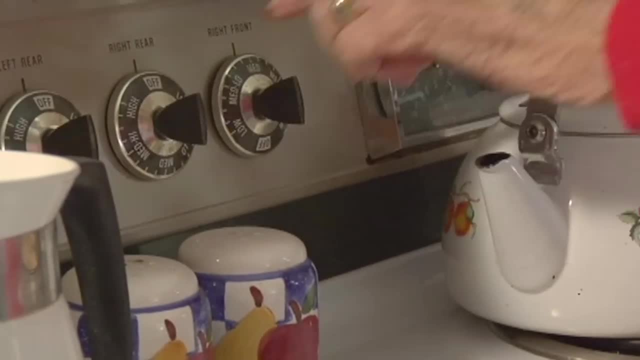 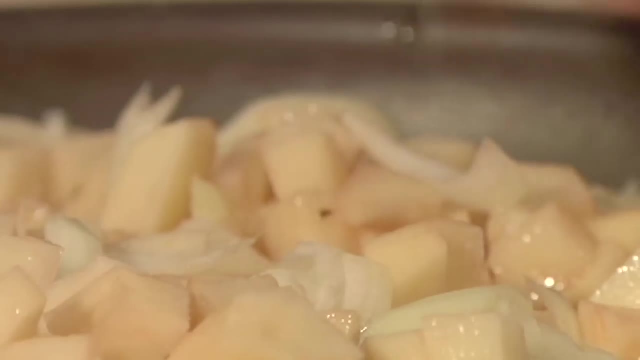 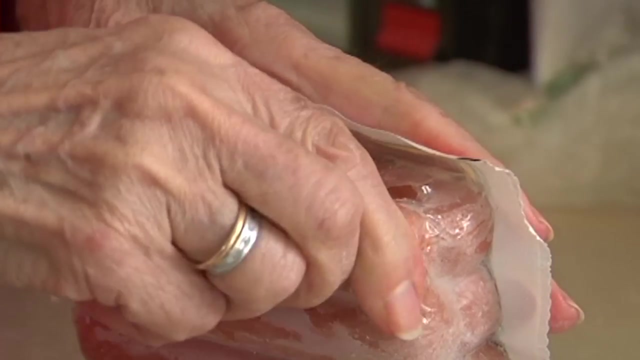 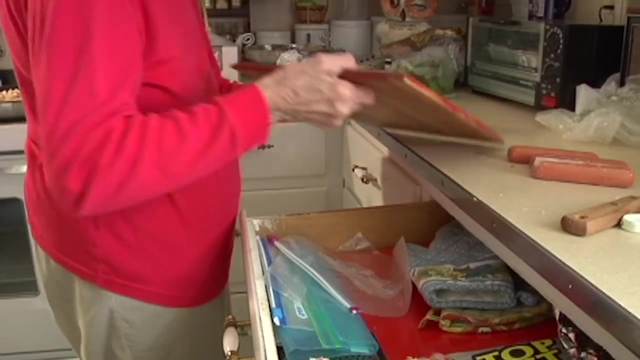 I got all the neighborhood kids coming in. They come in and they say: can we have the poor man's meal? They all liked it And we made up that name: poor man's meal. We should have called it the depression meal. 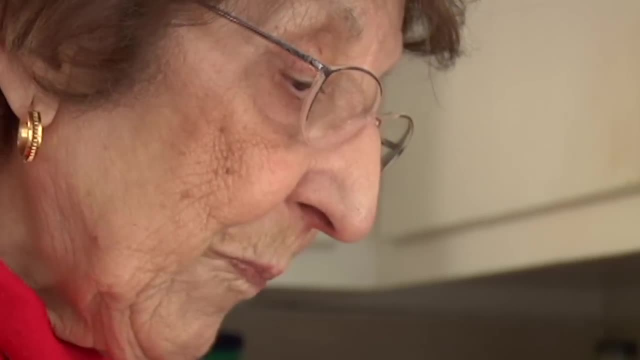 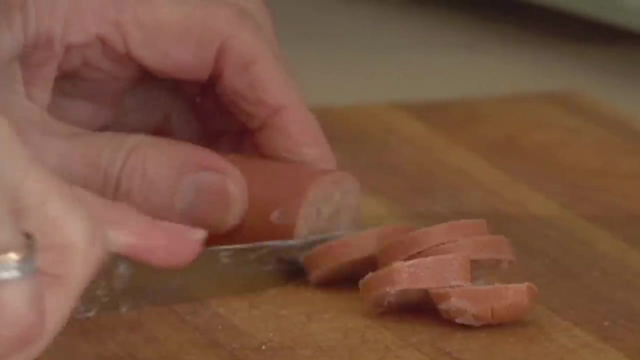 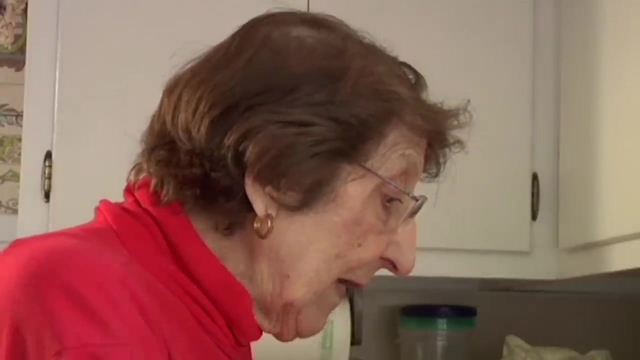 Getting the hot dogs ready, cutting them up so we could fry them with the potatoes, So we can fry them with the potatoes. It all depends on how many potatoes you've got. I think about four is enough for this amount of potatoes. Hot dogs are half cooked and they're tasty and they were cheap. 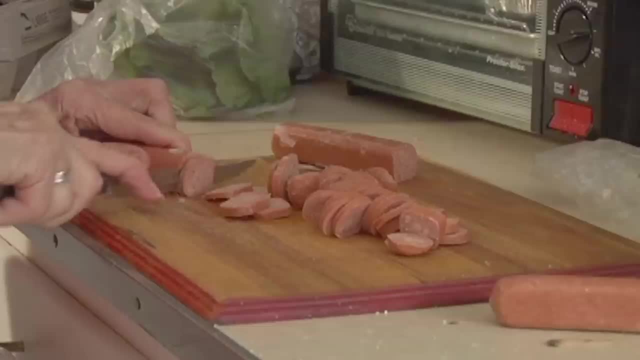 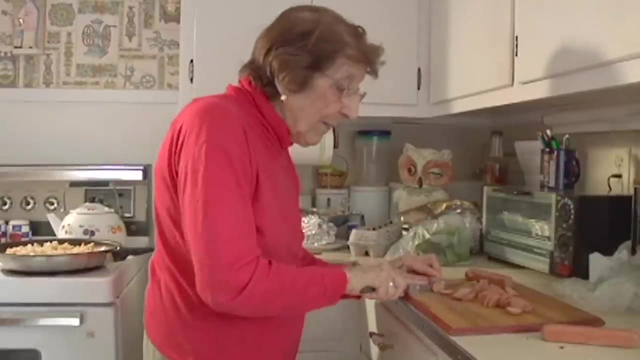 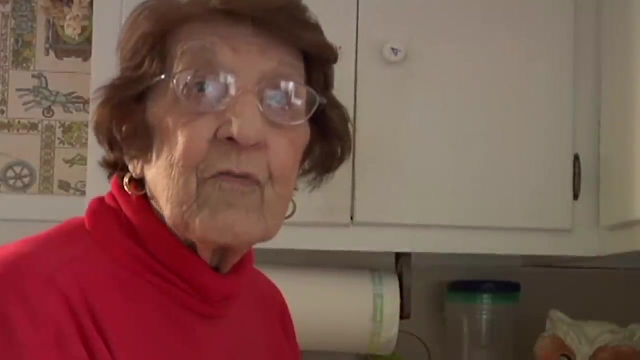 So anything that was cheap stick in. Oh, it's cold. Mark comes over. Nana, make me the poor man's meal. Then he brings his friend Tom. I usually cook for Mark's friends, their boys. They like my poor man's meal too. 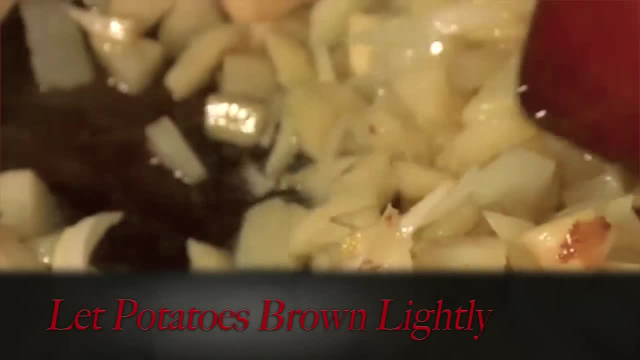 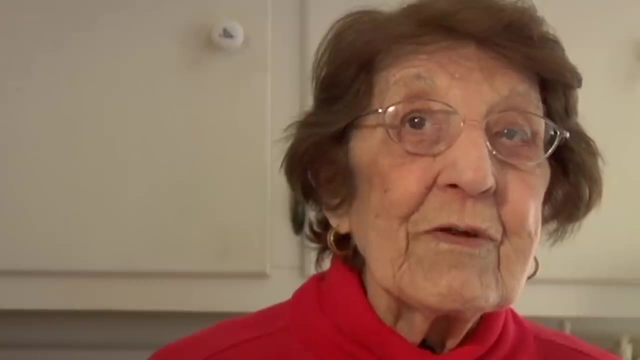 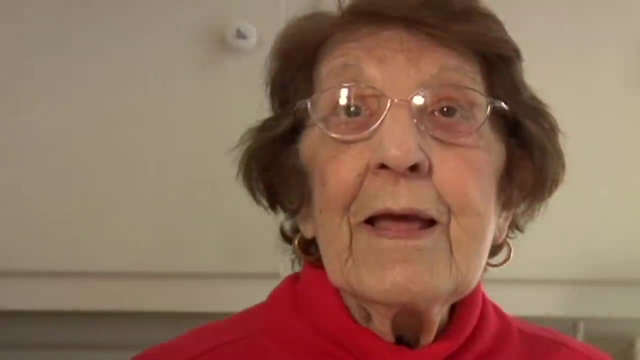 Starting to fry now. The pressure was very bad. it was a long one too. I had a little garden of my own. I had a garden of my own And a lady came- one of my neighbors- with a shopping bag and she was going in my yard. 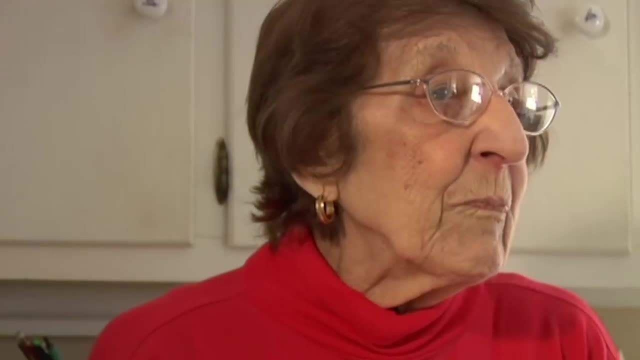 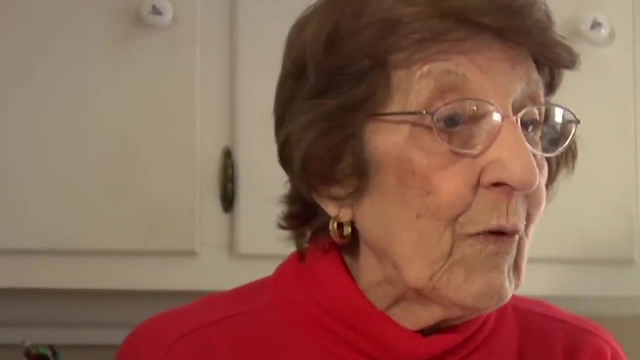 my garden And I said: where are you going? She said I'm going to pick a few things. I said: well, why don't you ask me? I'll give them to you, you know, but I don't want you to go there and just take what you. 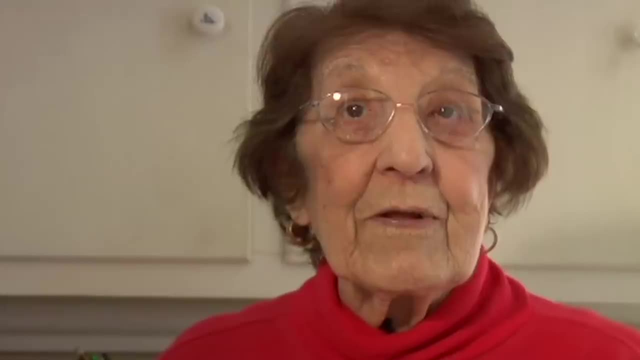 want. I said that's a lot of work for me. She was. she came to fill her shopping bag with my garden. Oh, I didn't think you were so touchy. I said I am touchy. I said no, I'm not touchy. 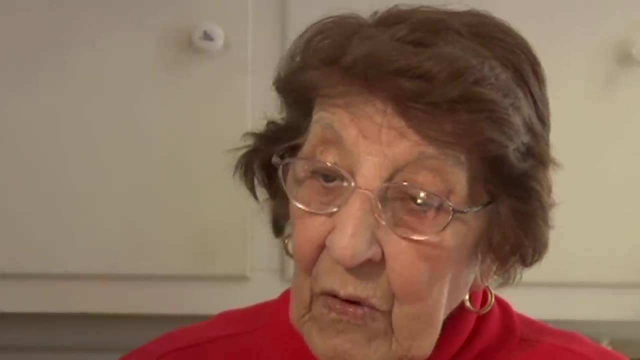 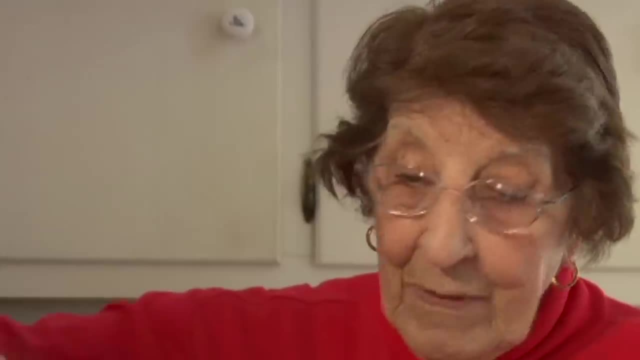 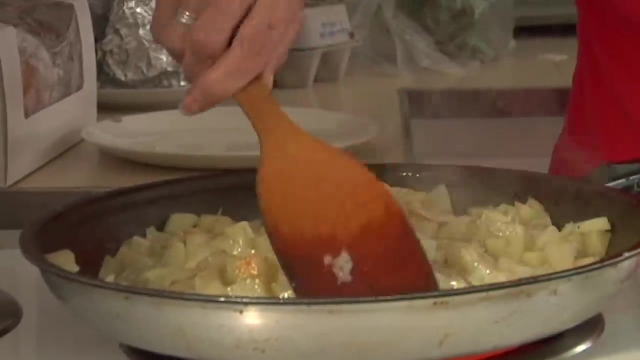 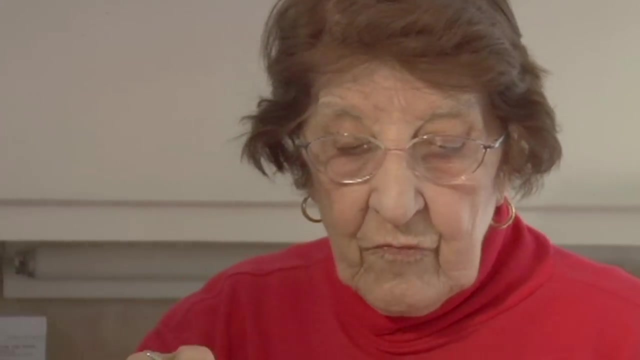 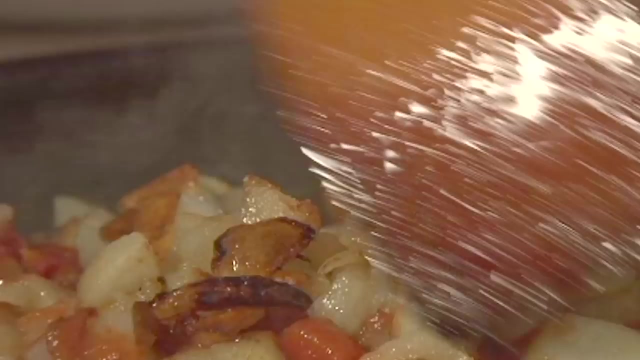 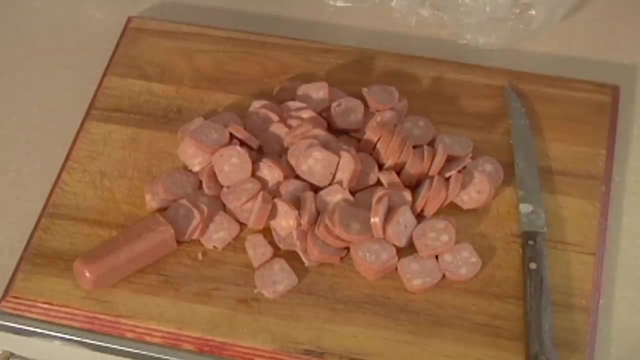 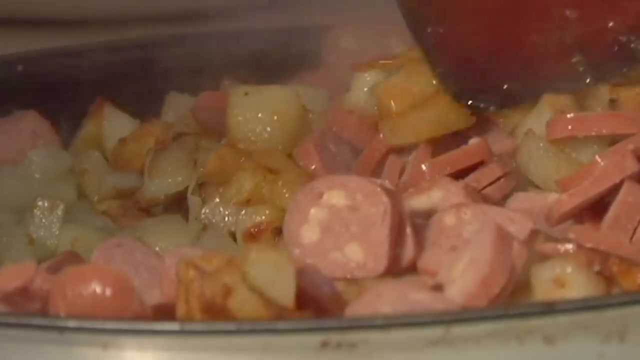 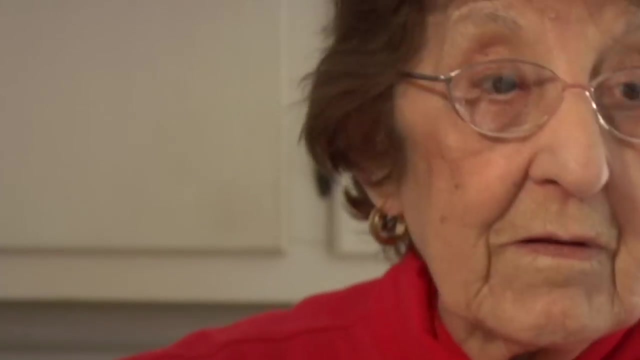 She just made herself at home. I'm going to put just a couple of tablespoons of sauce in here. Look at that. Look at that. I'm going to put the hot dogs with the potatoes. Taste the potatoes. If they're cooked, then you know they're done. 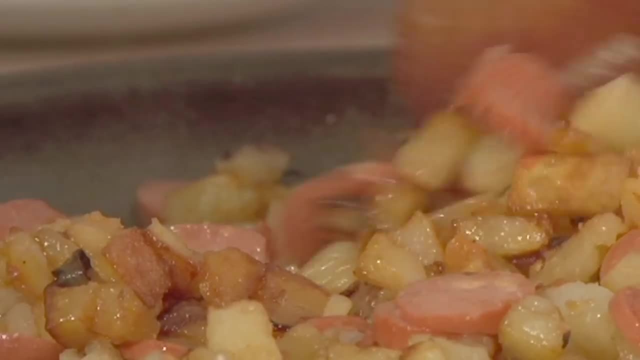 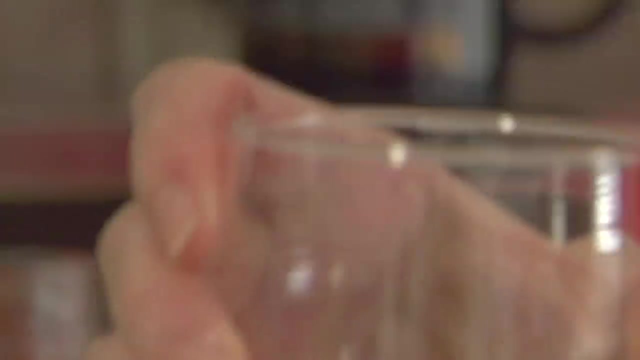 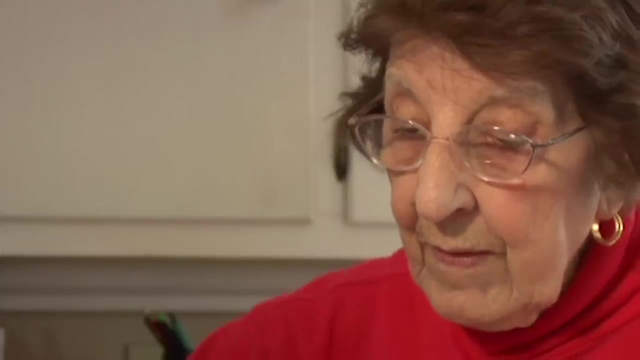 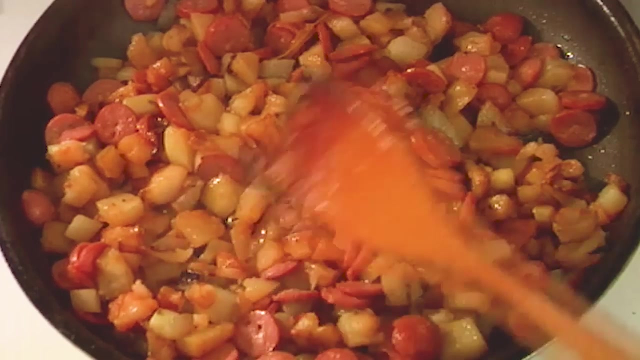 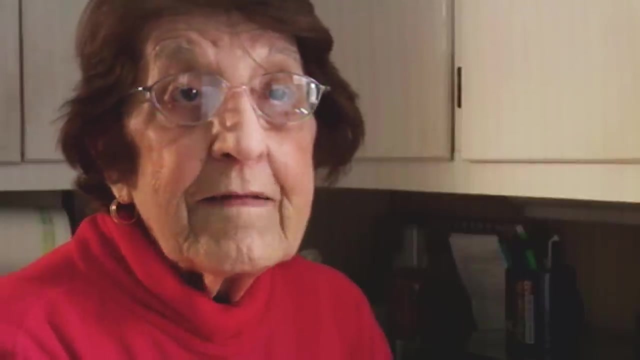 Hot dogs will get a little crooked- Well, those kind of bend. I put the water in so the potatoes will soften up and make a nice sauce for them. Let it cook for a few minutes and they're almost ready to eat. It has potatoes and hot dogs, so that's about it.